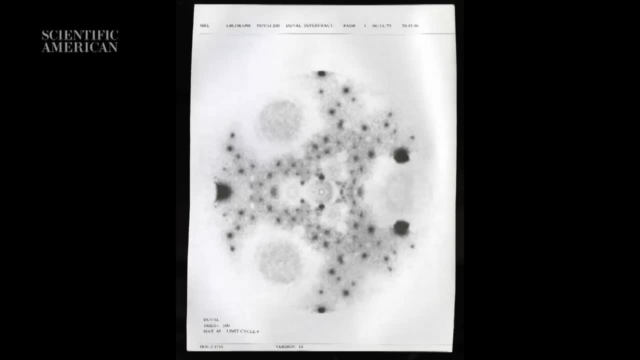 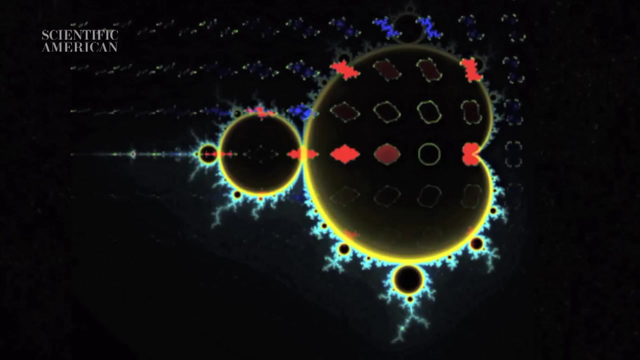 through visualization. Some experimental runs through the computers produced shadowy figures, some of which resemble shapes from the yet-undiscovered Mandelbrot set. Each image provided patterns for Mandelbrot to pursue and decipher, ultimately informing him how to adjust the data input. 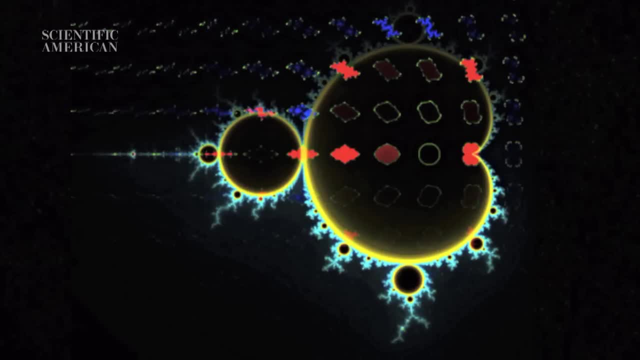 The Mandelbrot set is a mathematical set of points in a complex shape. It is related to other complex shapes called Julia sets, superimposed here in red. The limited power of computers at the time stymied Mandelbrot's efforts to understand the universe. The Mandelbrot set. 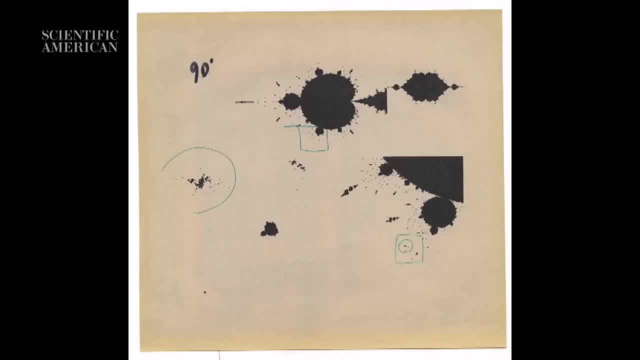 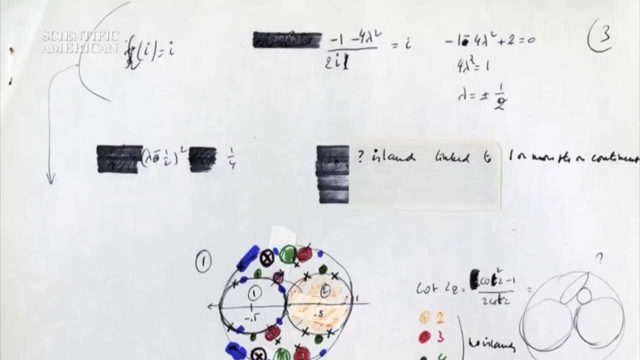 was used to calculate the finer details of the set. Here we see instructions to investigate speckles surrounding the set, something he referred to as islands. While Mandelbrot thought in rich visuals, this is one of the very few drawings in his hand detailing his quest. 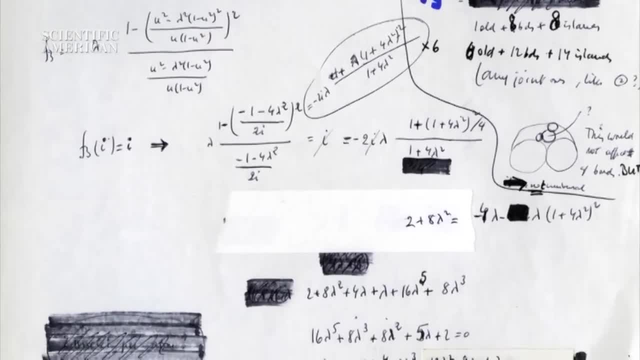 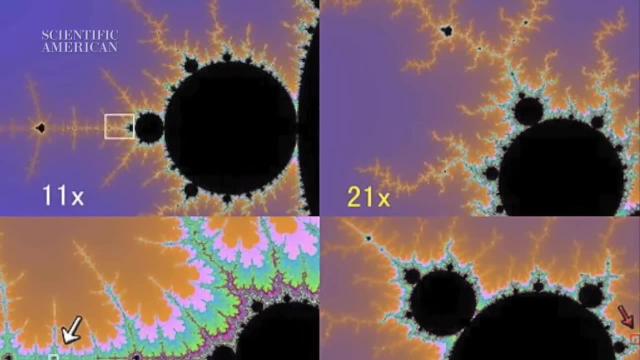 to determine if the islands were actually connected to the larger set. Ultimately, mathematicians Adrian Duotti and John H Hubbard would prove that the term island was a misnomer and the dots were in fact islands. They were not just small islands, but larger sets of patterns. 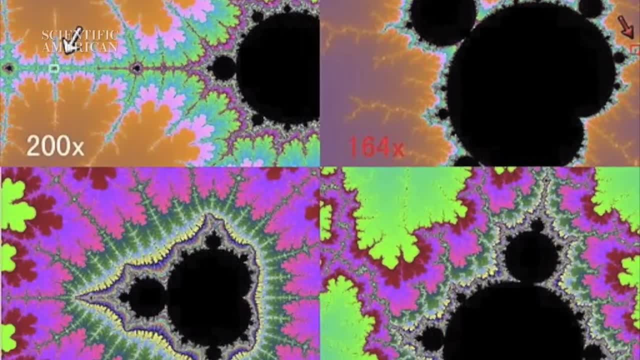 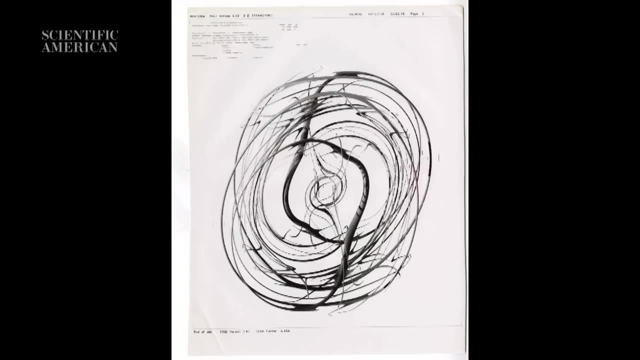 part of the whole. Mandelbrot also investigated other fractals and was interested in chaos theory, the idea that small initial differences between two dynamic systems could result in drastic differences over time. This image shows an attempt to visualize the dimensionality of such chaotic systems. 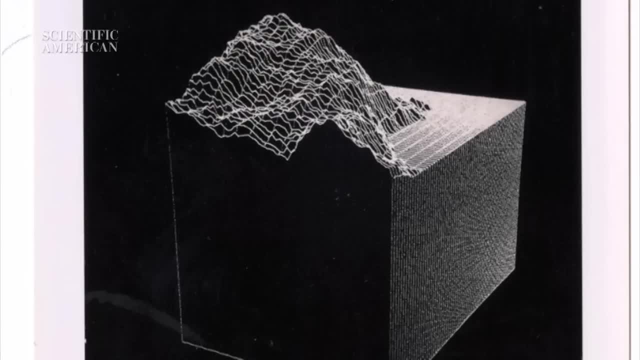 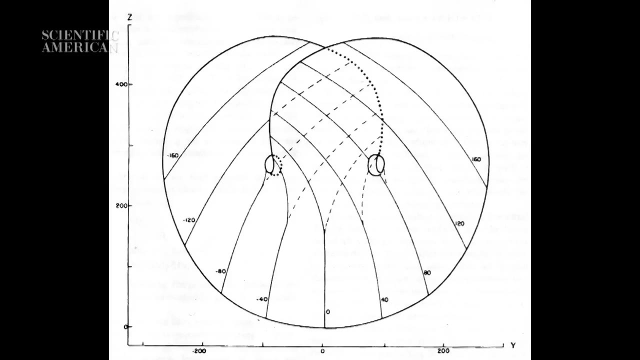 The complexity and apparent randomness of fractals can be used to create artificial landscapes, such as this mountain, that mimic the natural world. Visual representation of math can be more than just beautiful or illustrative. Here is a chaotic system known as the Lorenz attractor. It was first published. 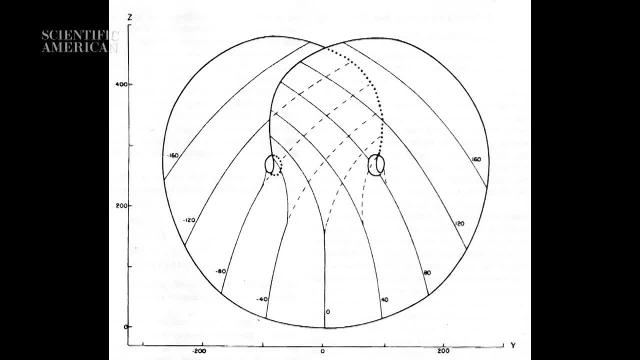 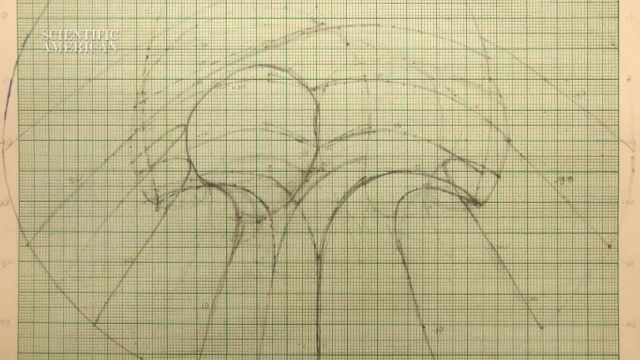 by Edward Lorenz, a mathematician, meteorologist and pioneer of chaos theory. Nina Samuel describes the system as existing between two geometric dimensions, but the flat image does little justice to this idea. This image is the same attractor, drawn in Lorenz's hand With pencil on paper. the scientist 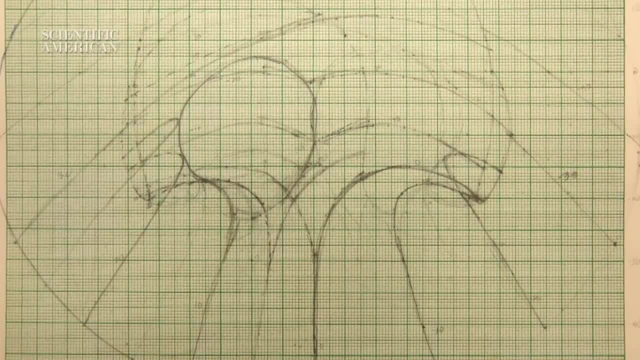 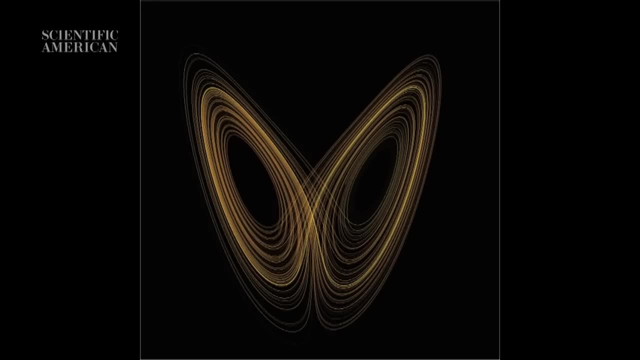 explores the shape of the attractor and the size of the attractor. The image is the shape and its characteristics. In this way, theory emerges through the process of drawing. according to Samuel's research, Now, with advances in computing power and technology, the chaotic system's shape can be more clearly.